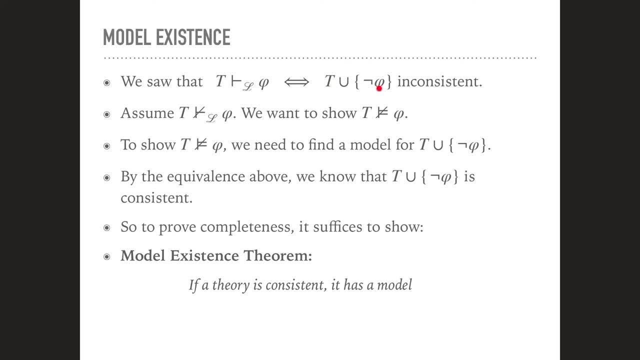 phi is inconsistent. So if I add not phi to the theory t, or rather the universal closure of not phi to t, then this becomes inconsistent. Assume now t does not prove phi. We want to show then, because that's the direction of the incompleteness theorem we want to prove. 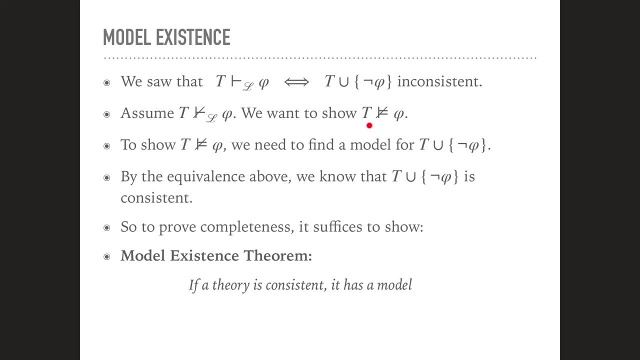 by counterpositive. So we want to show that t then does not logically imply phi. To show this we need to find a model for this set or this theorem. So we'll use the theory here- t union, not phi. Because if we can find a model for this, 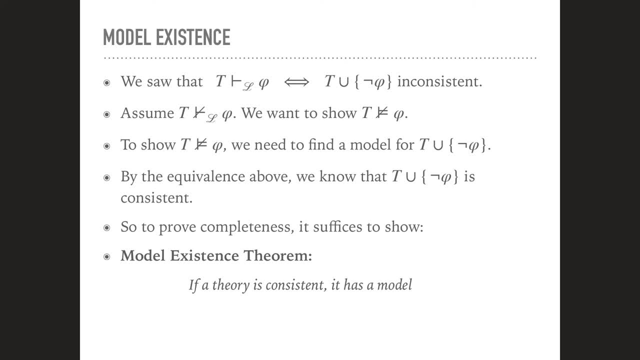 then that means that this logical implication does not hold By the equivalence above here. so by this equivalence, however, we know that t union, not phi is consistent, because we assume that t does not prove phi. So to prove completeness we can use the model existence theorem. So the model existence theorem. 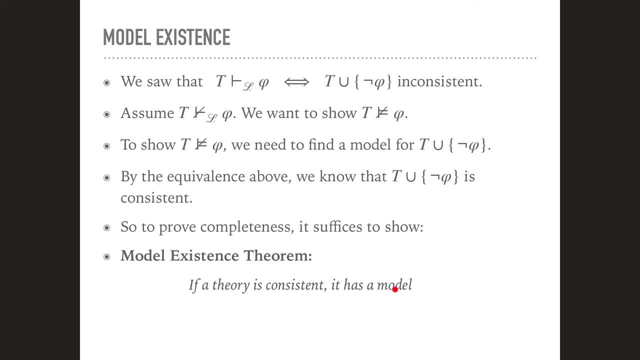 suffices to show the model existence theorem. If a theory is consistent, it has a model. So then we could apply it to this theory here and we would get that it has a model. So we would know that t does not logically imply phi. 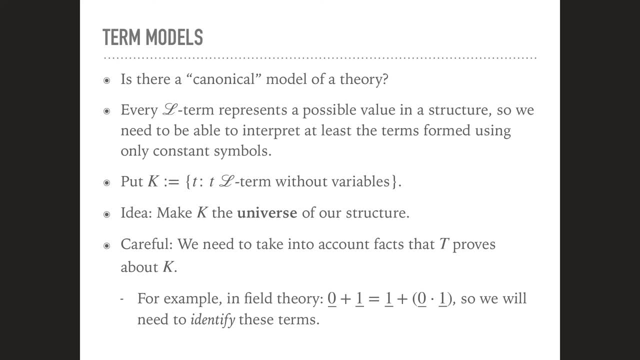 The big question is now, of course: is there a canonical model? pretty much out of the blue, because all we have is really the theory. In particular, we can ask: is there a canonical model of a theory? Well, if you think a little bit about it, we know that every l term represents a possible value in 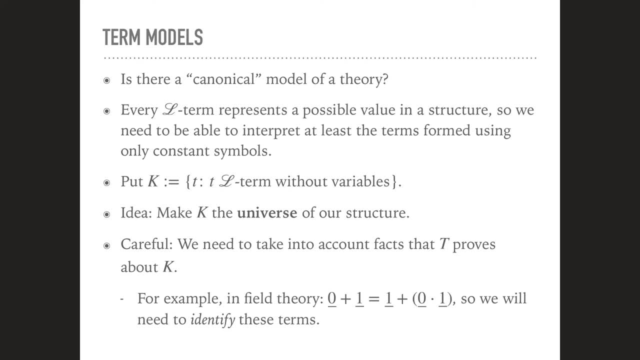 a structure. So if you want to give a model of a theory, you have to at least be able to assign every term a value in the structure, Right? So we need to be able to interpret at least the terms formed using only constant symbols. 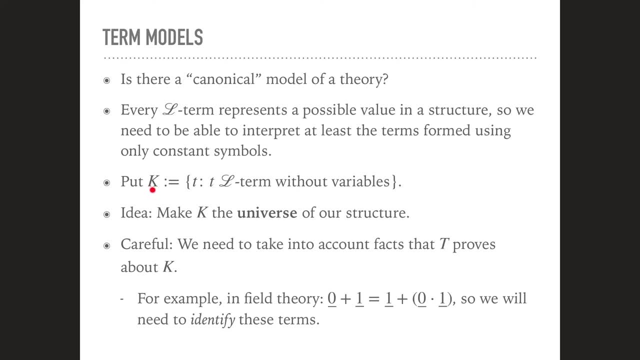 So let's collect those terms in a set. Let's call that set k. So k is the set of all l terms that don't have any variables. And then the idea would: be well, we need to interpret these, be able to interpret these terms right in a structure. So why not? 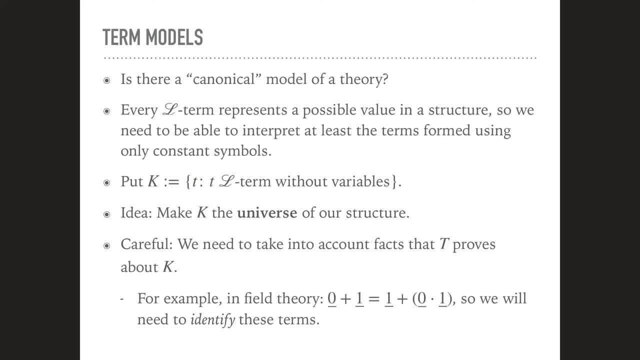 make these terms our universe right, So we don't even have to worry about what should be our universe because we need to interpret them, these terms. so why not let them be our universe right away? Well, we have to be a little bit. 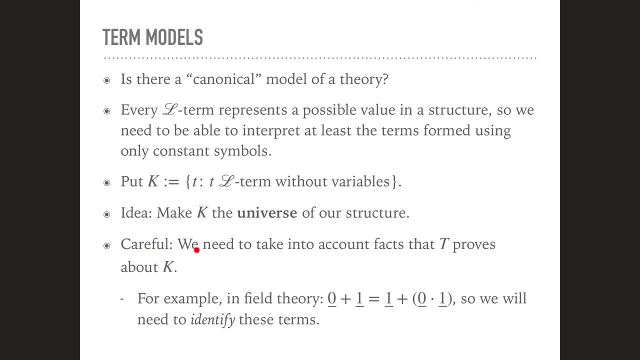 careful, not so fast. we can say here We need to take into account facts- that T proves about K. So for example, in field theory we can prove that 0 plus 1 is equal to 1 plus 0 times 1.. So these are both terms on the left side and the. 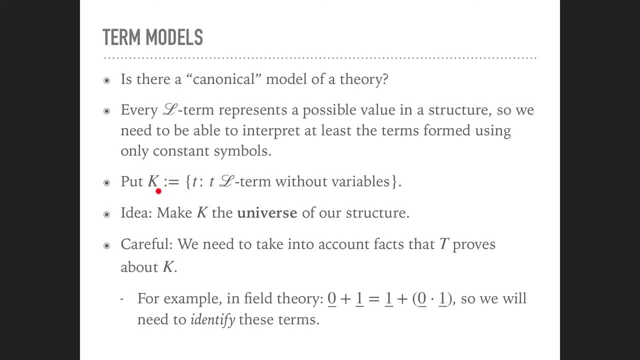 right side that don't feature any variables, so they would be part of this. set K here. But the theory of fields: right from the field axioms, we can prove that these terms actually are equal. So in our intended universe we need to identify these terms. So let's. 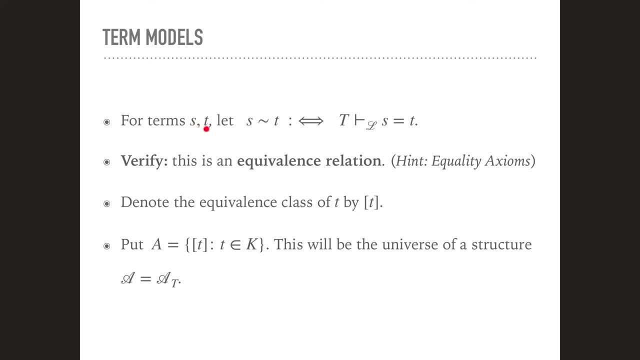 do that. So for terms S and T we say S is equivalent to T, even only if T proves that S is equal to T. We first need to verify some functions of an equation. when we vertically and vertically approximate, That is by representing the expression further another equation than 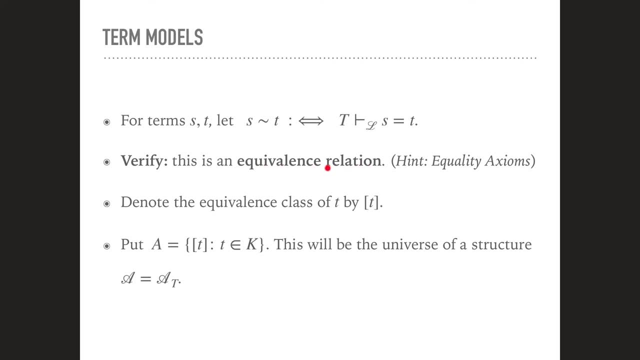 elsewhere, But this process ArchivesPflicht notwayswe are right Center data. It is like no erwarned- Вот je哦 쏘еж好 lee- when a particular byte has just been that this is actually an equivalence relation, and that's precisely what you. 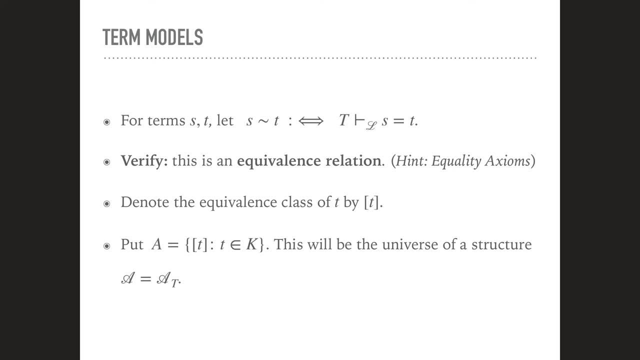 need the equality axioms for. So it's not hard: Take a look at the equality axioms and then show that this is indeed an equivalence relation. So once we know that this is an equivalence relation, we can take the equivalence classes and we denote the equivalence class of a term T by square bracket T. And now, instead of: 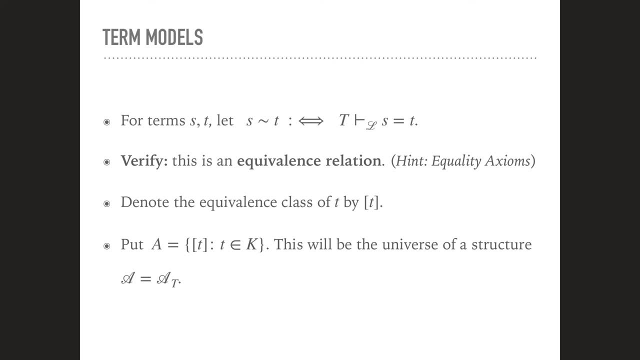 taking the terms directly, we actually collect the equivalence classes of a term in a set. Each term in K has an equivalence class and we collect that in a set A, And this now will be the universe of our structure, The structure A or also denoted by A sub T. So term models here refers simply to the fact. 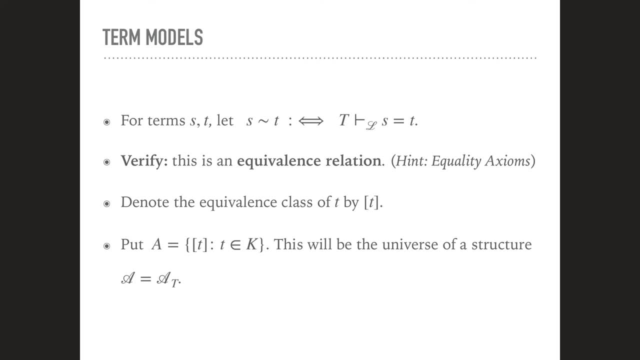 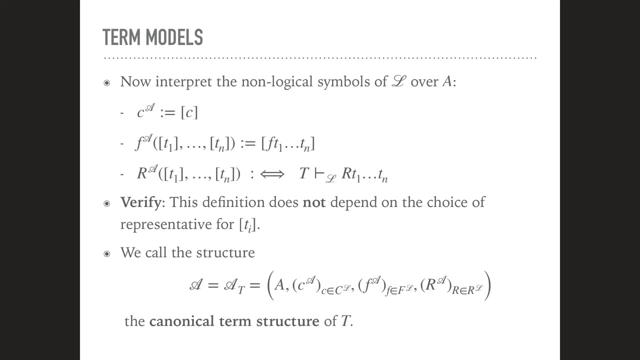 that the equivalence class is an equivalence relation. So this is the universe of our structure, will be given by the terms, or rather the equivalence classes of terms, Equivalence given by what T tells us it can prove about equality of terms. So now we have the universe of our structure, but in order 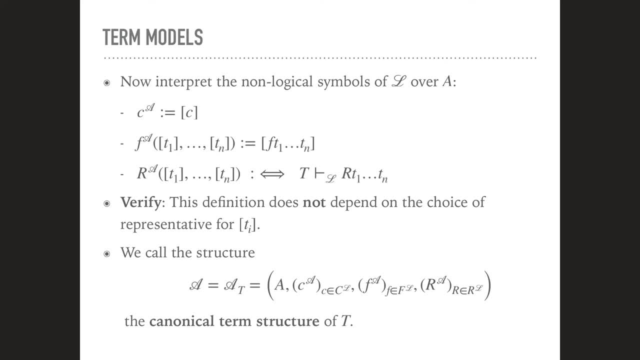 to make it a full structure of our language, we also need to interpret the non-logical symbols of our language over this structure And the way we set this up it pretty much suggests itself how we should proceed here. So, first of all, of course, every constant symbol interpretation. 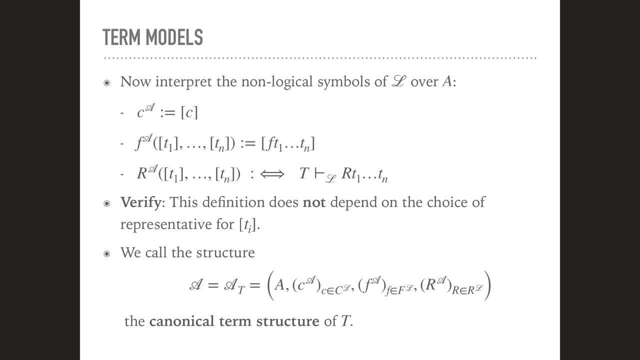 should just be the equivalence class of that constant symbol. Similarly, we need to define what the application of a function symbol to elements of our structure is. The elements of our structure, keep in mind, are equivalence classes of terms, And this is just a more simple example of how we can use this practice in the future. 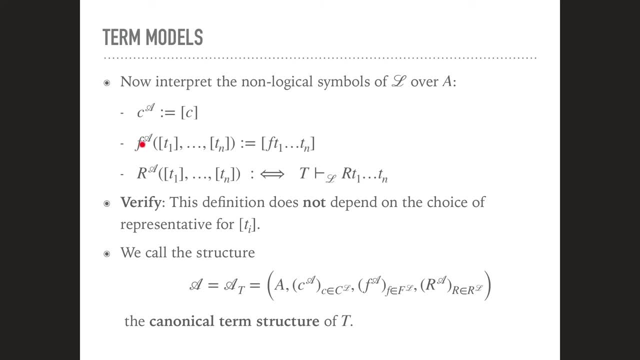 So what should the application of a function symbol f be right? Well, that's just the equivalence class of the term f. And finally, right for relation symbols. right, when should the relation r hold between equivalence classes t1 to tn? 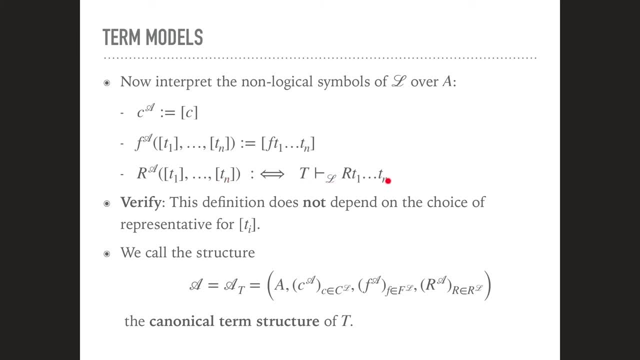 Well, it should hold precisely when t tells us it holds, namely if it can prove that this relation holds between the terms t1 and tn. And you already see here, this might actually be a problem later on, because t might not actually be able to be expressive enough. 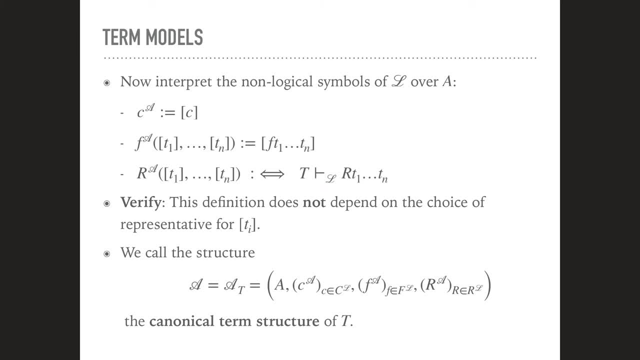 So this could cause problems down the road And t might not be powerful enough to settle all the relations, so we might actually miss defining some relations that we should down the road. So this foreshadows a little bit what we'd have to do later about t. 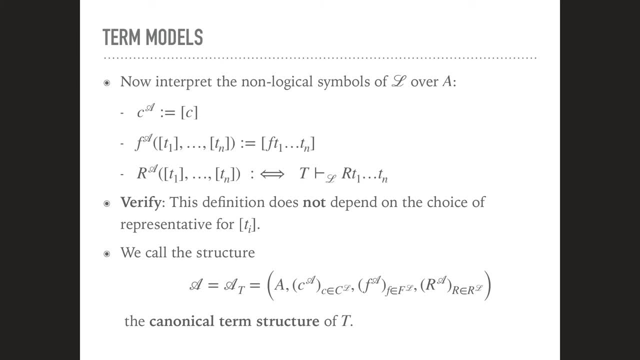 But we'll get back to that in a couple of slides. So now we need to verify that this definition does not depend on the choice of representative for each equivalence class here. right, Because we're actually using the representative here to define, for instance, the value of 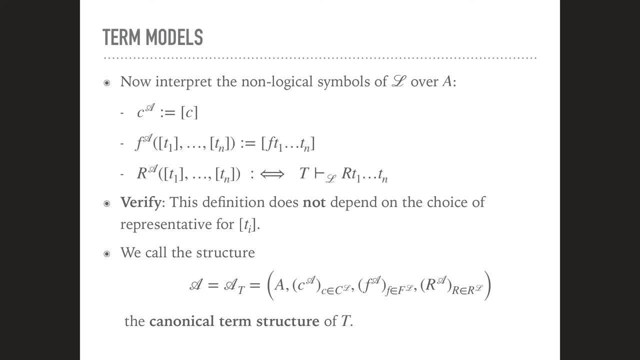 this function application here And again, just as before, you take a look here at the equality axioms, right, Remember, these equality axioms also included the congruence for functions and relation, and that's precisely what you will need here. 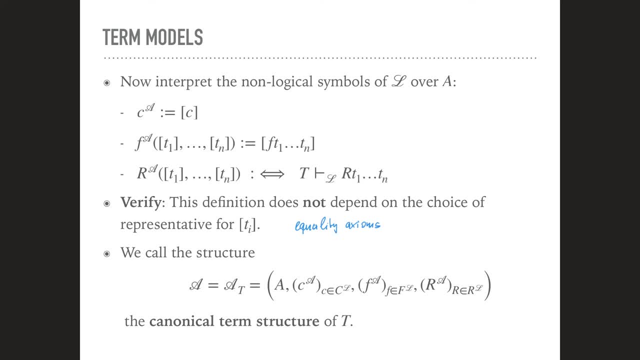 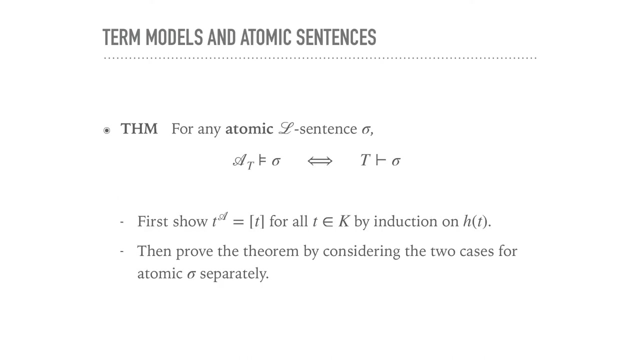 So, once you've verified this, we actually see that all these definitions, then, are well-defined. We get a structure, And this structure that we get this way we call the canonical term structure of a theory, t. So we now have a structure. 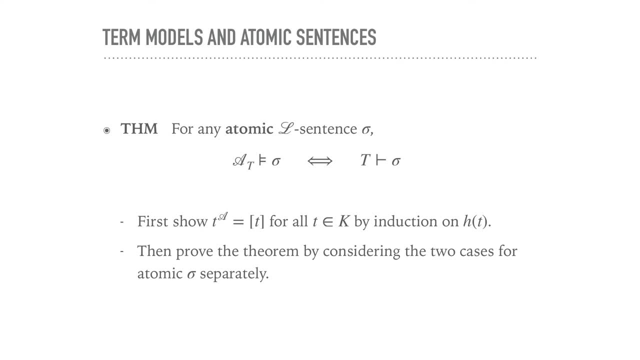 A structure defined that is somehow related to t, And the hope is that this structure a sub t, so the canonical term structure would be a model of t. And if we were only concerned with atomic sentences, that's actually true because it: 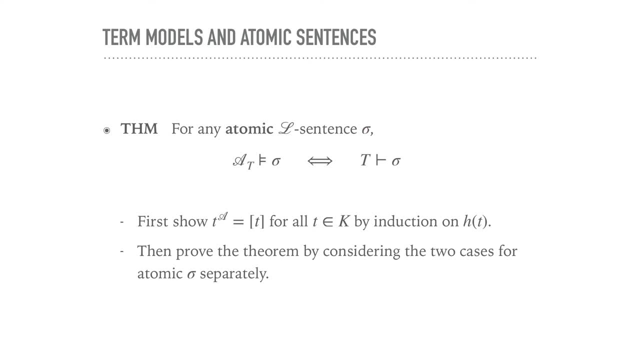 holds that for atomic sentences sigma, this sigma is true in a sub t if, and only if, t proves sigma. So for atomic sentences a sub t is a model of t And you show this by first showing that for every term, the interpretation of that term. 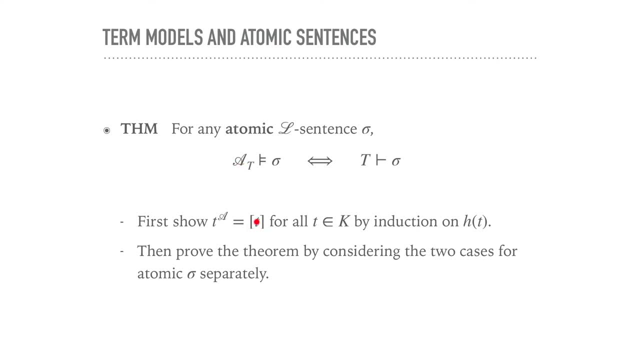 in our canonical term, structure a is just the equivalence class of t And you show that for all t in k And as usual you get a model of t. You show it by induction on the height of t And then you prove the theorem by just considering the two cases for atomic sentences separately. 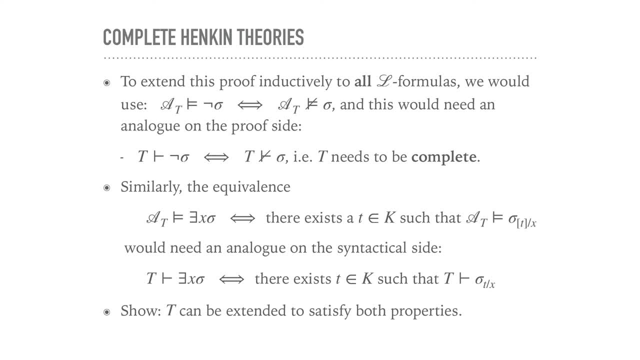 Of course, we would like to extend this theorem or this proof, now inductively to all l formulas or l sentences. Well, we would use, for instance, this: This is the first case, This is the second case. For example, in the case of negation, we would need to use that at models, not sigma. 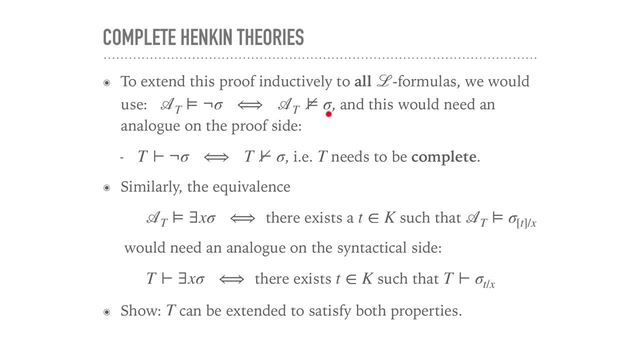 if, and only if, at does not satisfy sigma. But we would need to be able to connect this now to the proof side, So it would need an analog there, And that analog would be that t proves not sigma, if, and only if, t does not prove sigma. 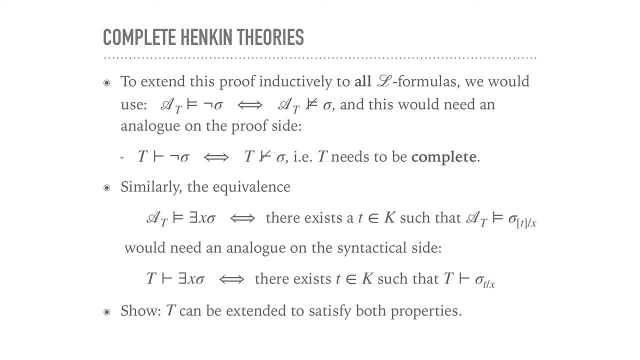 And that's precisely the property of t being complete. So, if you recall, complete theory, for every sigma it proves either sigma or not sigma. Now, similarly, the equivalence in the inductive step, we would extend in another inductive step to formulas with an existential quantifier. 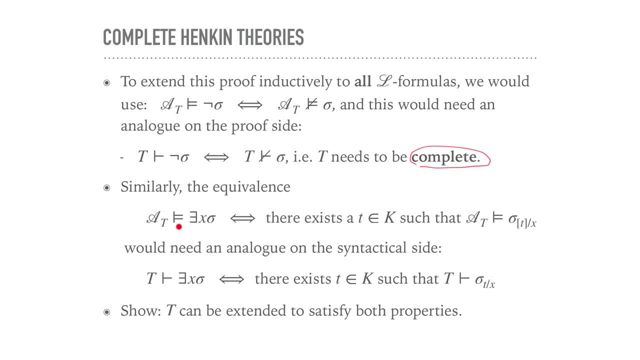 And here we would use the equivalence that at satisfies exists x sigma, if, and only if, there exists a term in k such that at satisfies, sigma. if I plug in, if I evaluate the variable x as the equivalence in class of the term t, 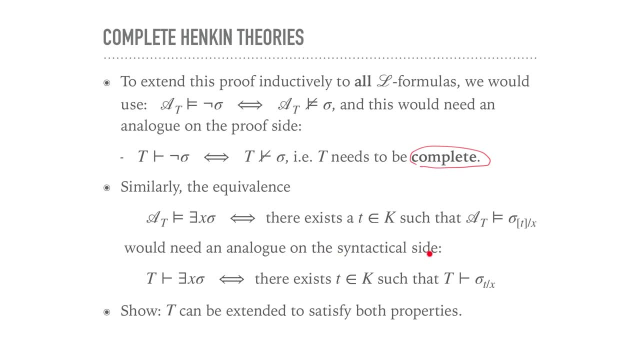 So this again would need an analog on the syntactical side. In that case it would be: t proves there exists x sigma if, and only if, there exists a term in k such that t proves sigma with t substituted for x. OK, 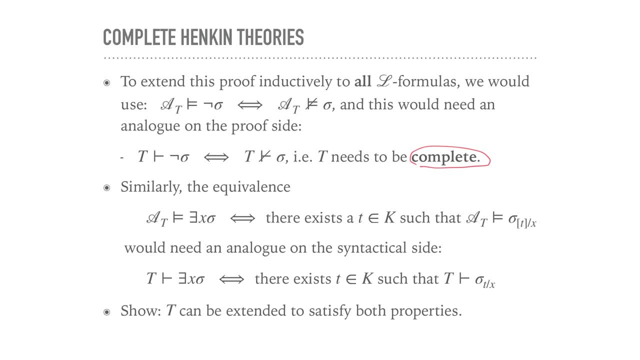 Theories with this property have a special name: They are called Hankin theories. So this is the so-called Hankin property And this will play a crucial role, as you may imagine, in the proof of the completeness theorem And what we need to show now, and that's the work ahead of us. 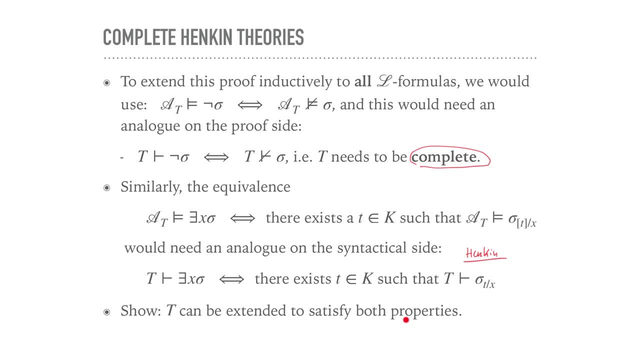 is that t can be extended to satisfy both of these properties without changing the proof of the theorem. So we can extend the proofability properties or consistency properties of t in any way. So that's the project ahead of us. Can we extend t to be complete and also? to have the Hankin property. Engineering is about problem solving, and modeling and simulation is problem solving on steroids. It's taking information from every field you could possibly think of and finding a way to model it mathematically and then create a simulation that will allow you to predict behaviors. It's a program that deals with creating models that simulate real life scenarios. 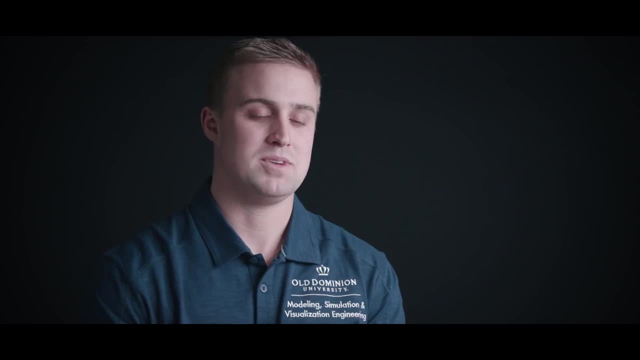 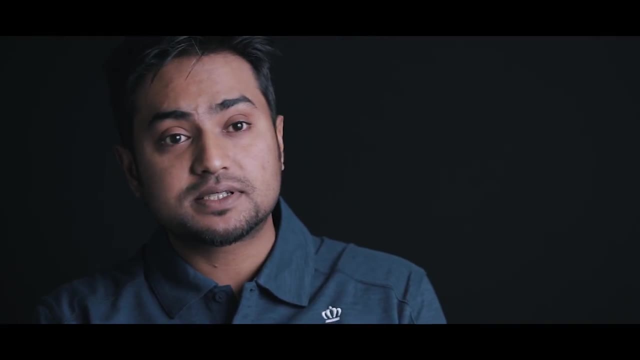 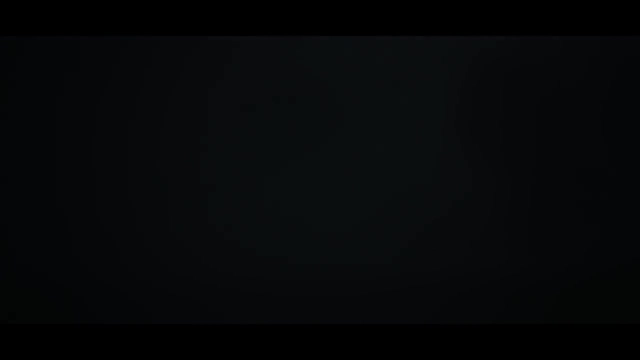 What our degree represents is the ability to take a problem and solve it in a way that very few people can. From transportation to cyber security, to healthcare system, robotics, game development platforms- you can use M&S anywhere. I am actually interning at NASA Langley Research Center working with developing augmented and virtual reality applications. 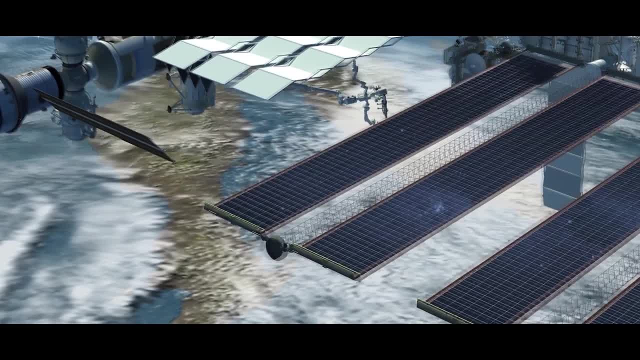 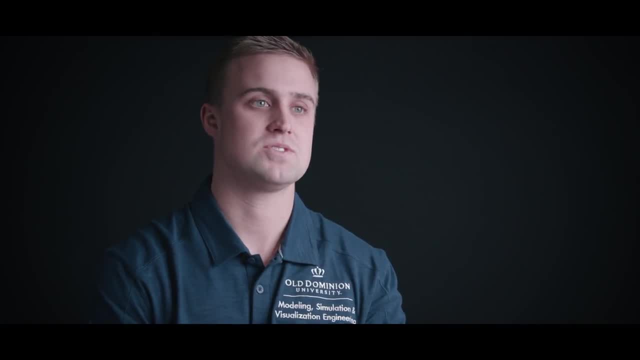 Some of the work we do is with NASA, and I've had the opportunity to work with them on the space habitat they're building. It's very interesting. We have a very specialized degree and we're the only institution in the country that offers an undergraduate in that degree. 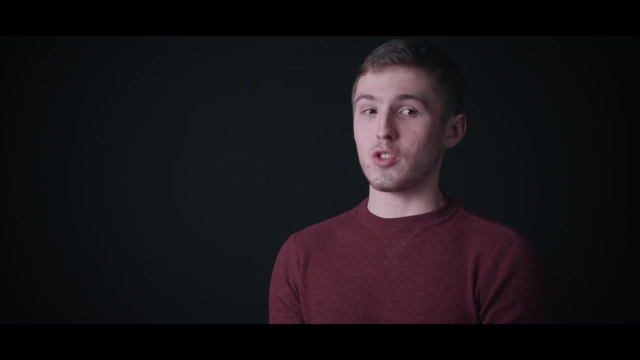 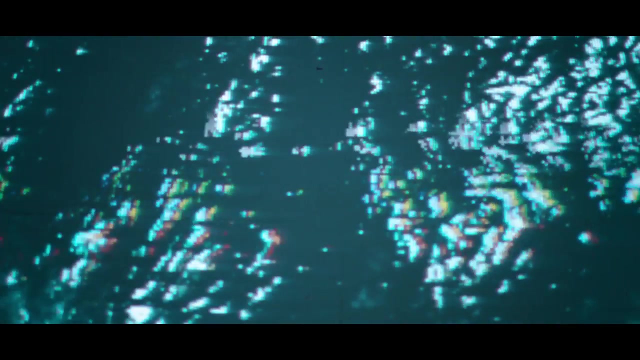 You're not only an engineer, you're a programmer. They're doing a lot of hands-on interaction with a lot of the different programs like ARENA and SIMEO, So you're not just knowing the math and everything behind it, you're actually getting to physically use these different programs and devices that you'll use once you're out in the workforce. 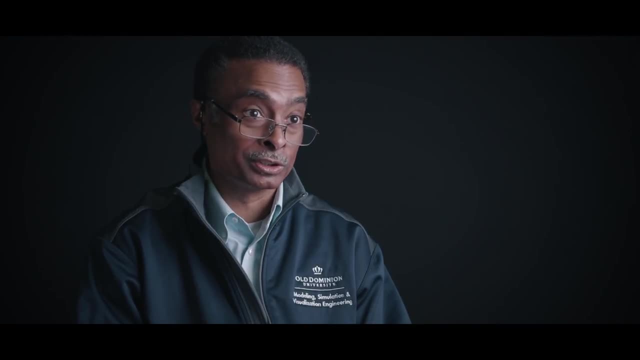 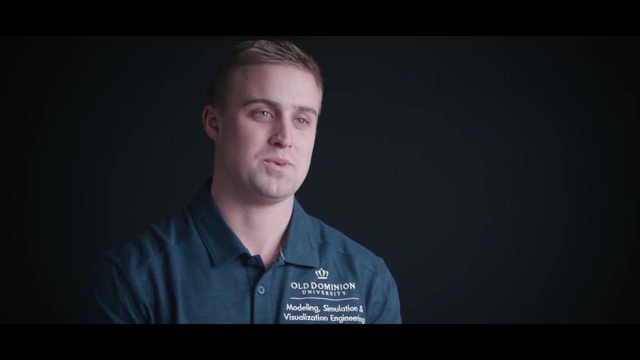 Many of our students have two or three job offers before they even graduate. I had a couple job offers while I was still in school. I've transformed from a student who didn't really know what they wanted to do to having multiple job offerings and finding myself along the way and really nailing down and pinpointing what it is I want to do with my life. 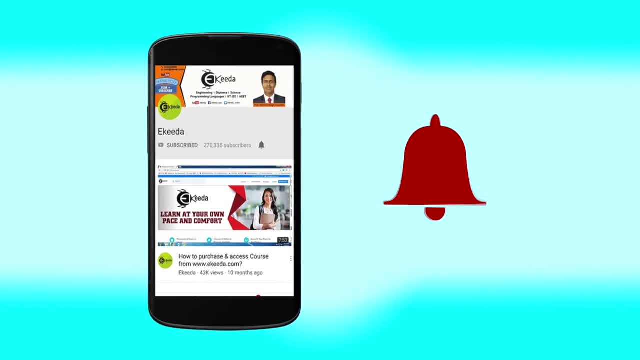 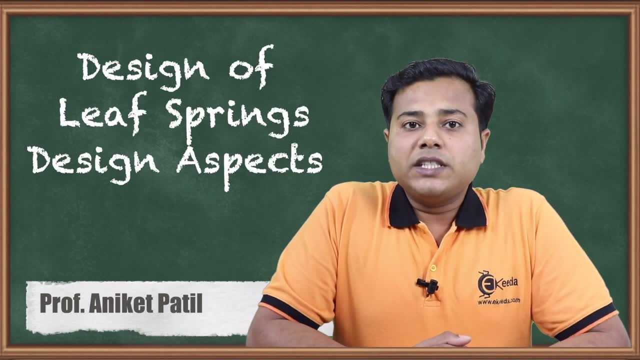 Click the bell icon to get latest videos from eKIDA. Hello friends, welcome back to the subject of Machine Design: 1. We are right now learning the module number 6, where different designs associated with different types of springs are learnt. In last session we have completed one numerical which is based on design of helical spring which undergo both static as well as the fluctuating loads.